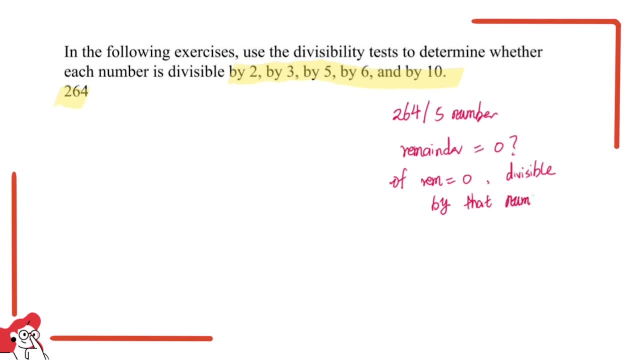 And otherwise it's not. Okay, so very simple, And consider it's a very long calculation. Okay, so very simple, And consider it's a very long calculation. And consider it's a very long calculation. We should go through this question together. 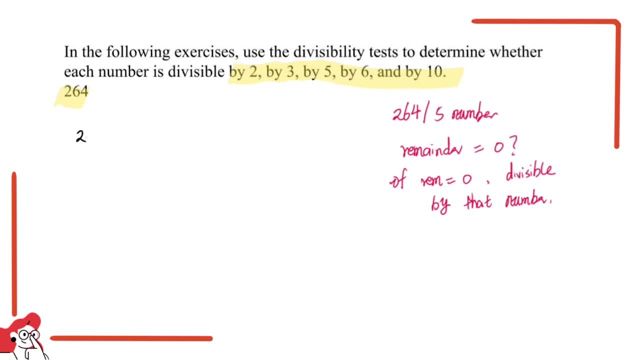 Okay, so we first do 264 over 2.. So we simply we should get 1 over 2, and we have 64.. So we should have 32 in order to have 64, and the remainder is zero. So two is then is one of the answer. 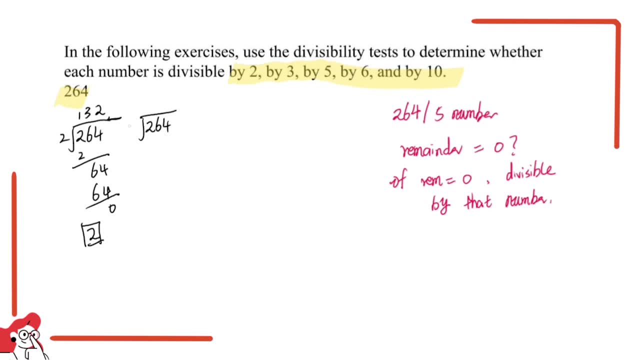 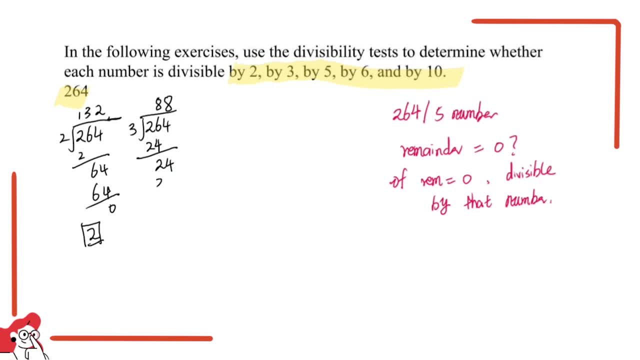 And what's left is 24 again. Now we just put 8 right here and we should have the remainder zero as well. And now we just put 8 right here and we should have the remainder zero as well. So 3 is another answer. 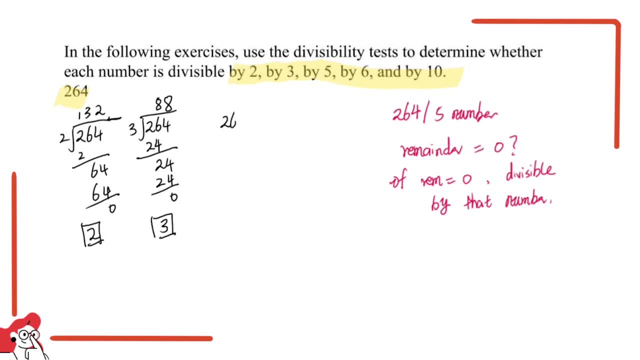 So 3 is another answer, And let's do 5 next, So 5.. So let's do 5.. So let's do 5.. We can multiply by 5. We get 24.. we get 25 right here. we'll slap this 14, and we can put 2 here, in order: 10 and 40 becomes 52.40. 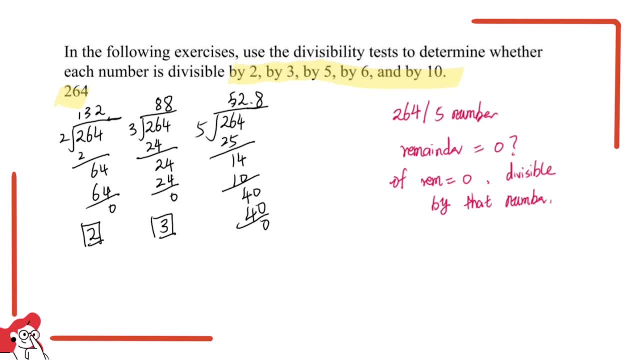 in order to have zero. uh, remember also sorry. although we can, we can divide this and we can get a number which is 52.8. however, it does not mean this is divisible and this is dividable by 5, because we need a whole number. okay, we need a whole number in order to say that 2: 64 is. 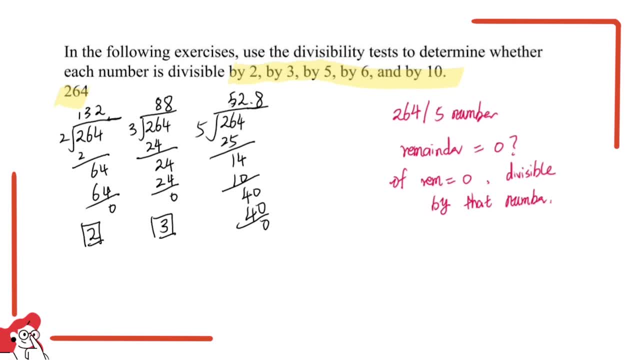 divisible by 5.. but right here we have, we have a decimal right here, so it's not divisible by this by five. okay, all right. next we test six, so we can put a four here. so four times six is equal to 24.. and we'll have 24 again. so we just 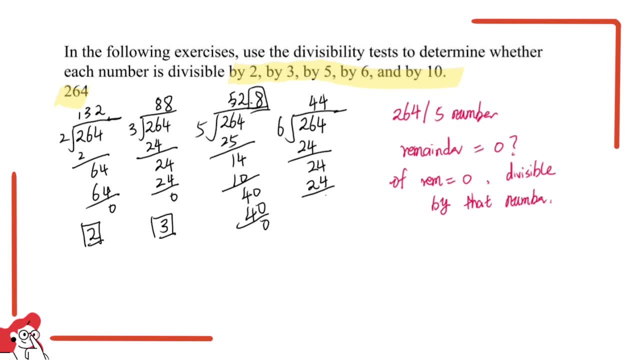 put six right here, so 24, and this equal to zero. so six is another number, is another answer. and last we have 10.. well, it's very easy to do this, because two sticks over 10 is equal to 26.5 point four. we just move the decimal place one place to the left and you get something like this: 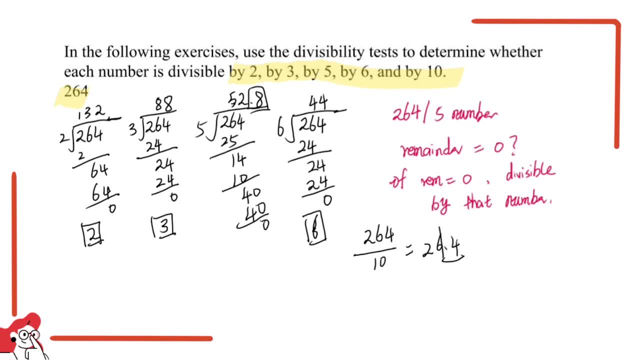 and also we can see that it's not a whole number. we have a decimal right here. so let's say that 10 is not one of the answer. so 264 is not divisible by 10.. okay, so only whole numbers. so the answer has to be: all numbers has to be. 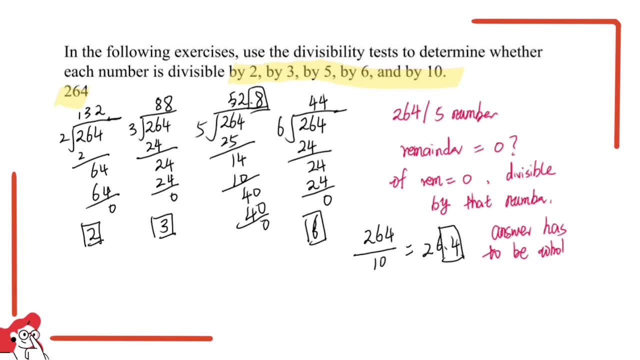 all numbers or integers, right to be more specific integers. integers, okay, in order to be, in order to let. 264 can be divided by that one, okay, so two, three, six and four, i'm sorry, two, oh, this is very, very missed, very easy to misunderstand. so 264. so we should have a circle on the line right here. 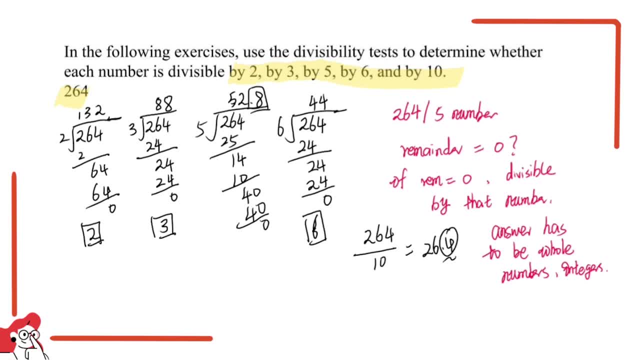 okay, so from the question we know that two, three and six- these three numbers are the answers, and 264 is divisible by these three numbers- two, three and six- because after division was left it, which means the remainder is zero, and also the answer is a whole number. so 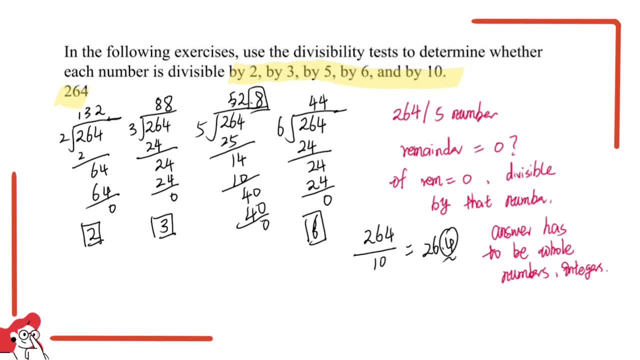 meeting these two conditions means that it should be the answer. and what's the takeaway for this question is how to solve questions like this, how to determine whether a number is divisible by the other number. we just need to do the division and see if the remainder is equal to zero and if the answer is a whole number. that's the two steps, okay. 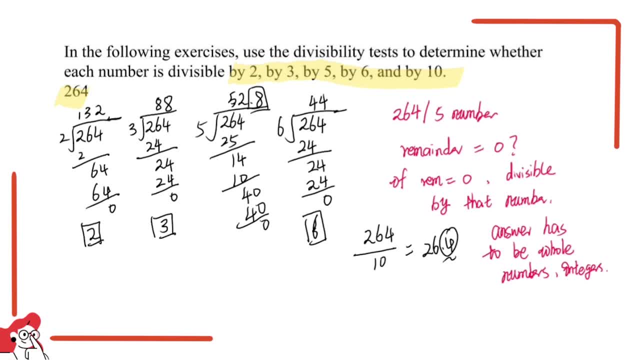 so that's all for this question. see you in the next video. you.